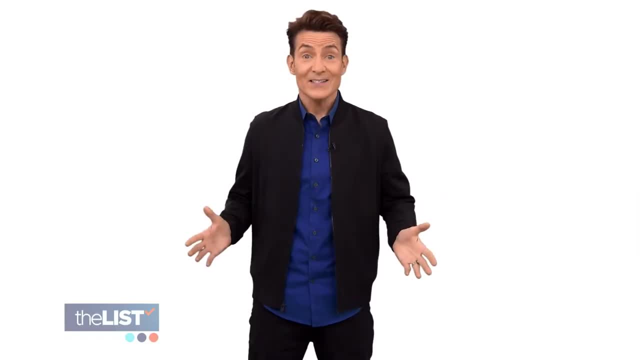 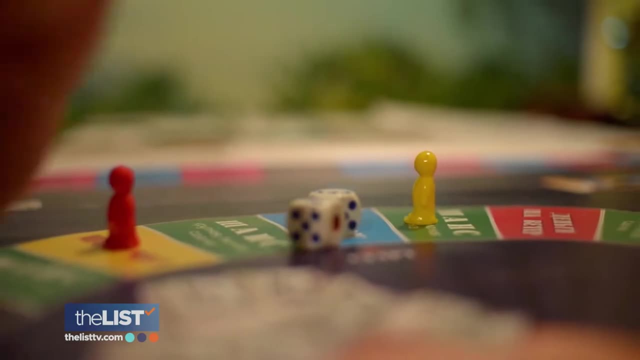 Oodles, Scattergories and Taboo. I have every single one of these on my shelf And let me thank you for your royalties, For your loyalty. Like writing a book, creating a new game is something a lot of people dream of doing. 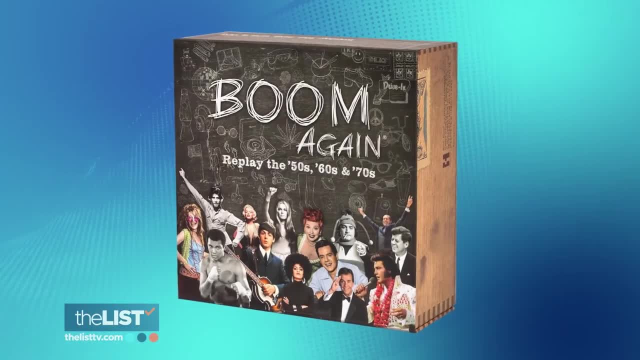 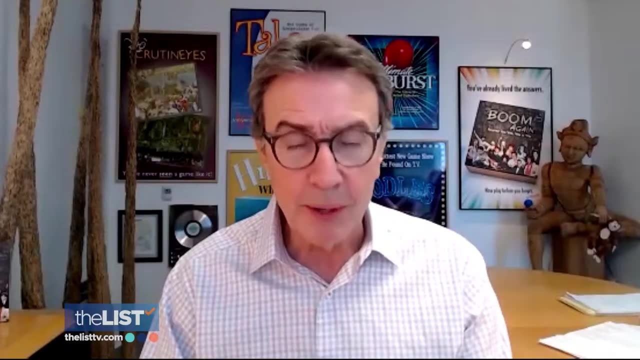 Even Brian, who's at it again with his latest party game: Boom Again. So we're getting pro advice on how to create a game For starters. set aside your nagging doubt and just dive in. Just do it. Sit down, create your game, do it on paper, mock it up any way you want. 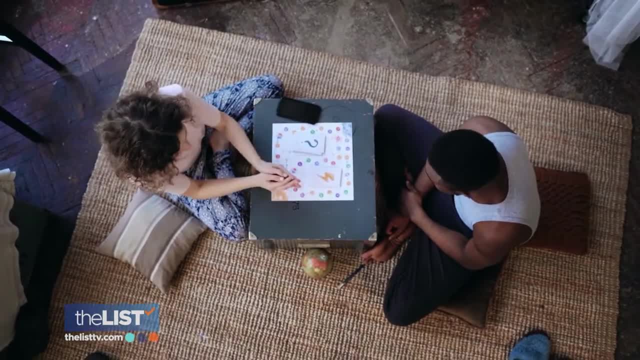 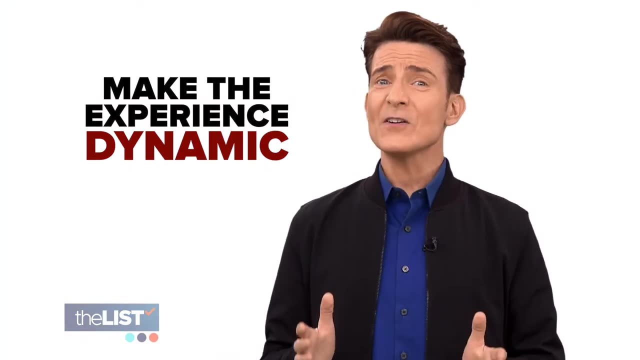 Just get the idea out of your head and into some physical format that people can play. When I made Taboo, the original buzzer was my garage door opener- And make the experience dynamic so you're not hitting the same note over and over. 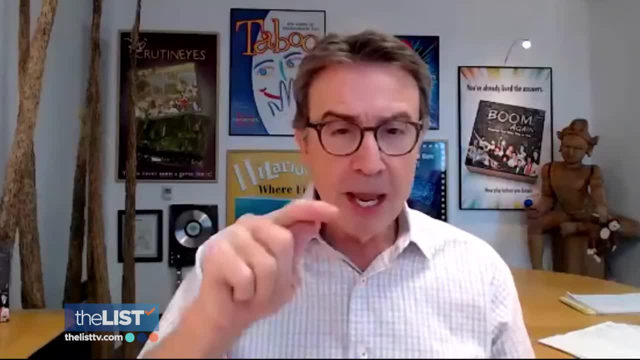 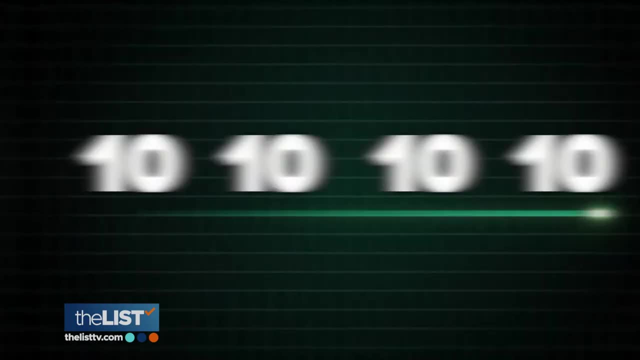 In the game Outburst we'll ask you 10 cars rich people drive. If you name all 10, that's a very high success rate. If you did that on every single question in the game, it's a flat line. So I want to have you get 10 and be thrilled. Then I want you to be frustrated. 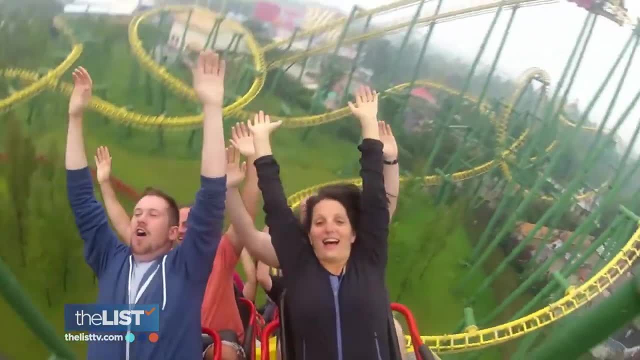 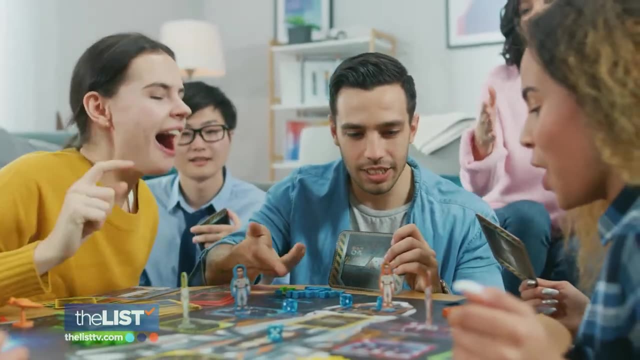 Then I want you to be excited, Then I want you to be angry. I want you on an emotional roller coaster. It's more fun. It's more fun than being on a merry-go-round. So sure, throw in some gimmies, but 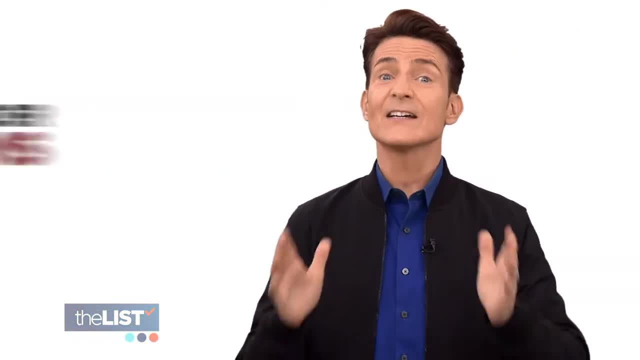 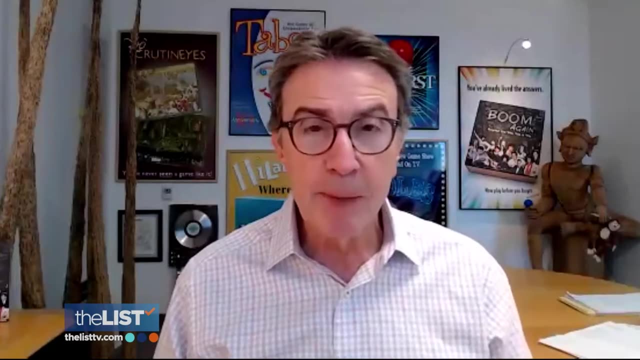 You also want people to suffer a little bit. Next, consider teams. If you have a game that's about drawing, you know some people don't like to draw. If you have a game that's about trivia, some people don't want to be embarrassed. 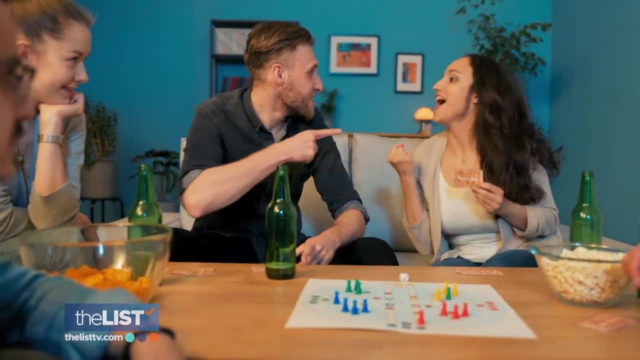 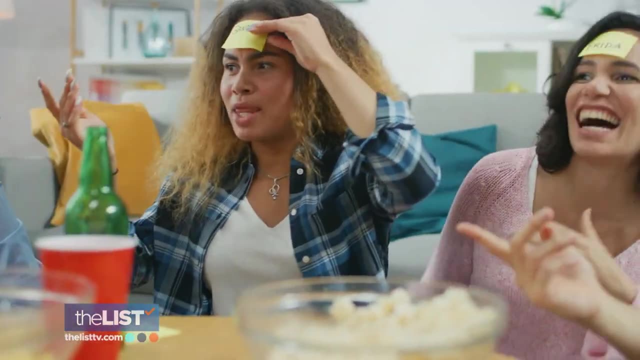 And teams invisibly deploy the enthusiasts to prop up the reluctant. It's really about the working together. I may know a piece of the answer and that may trigger you to know the rest of the answer. That's an easy way for us to work at succeeding and enjoying the game. 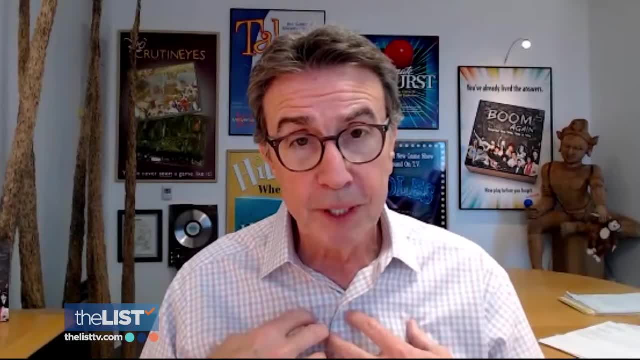 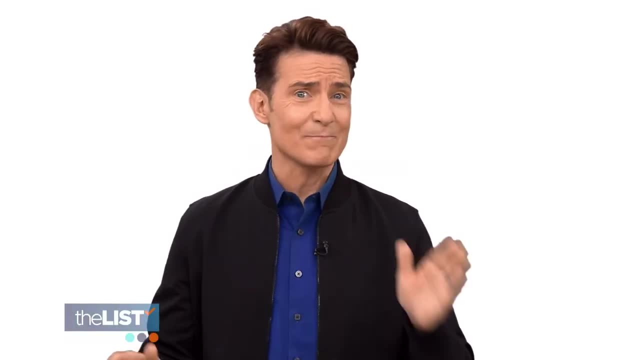 And it stings less to lose as a team. I don't want to look stupid individually, but if I'm on a team of imbeciles, that's okay. Hey, I'm the lifetime captain of team imbecile, Okay. so you've taken all this advice and mocked up your game into a crude but playable prototype. 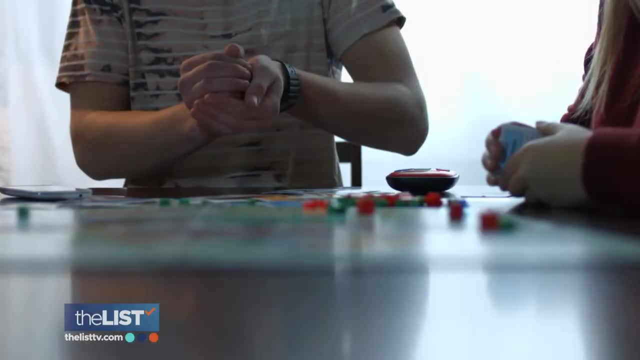 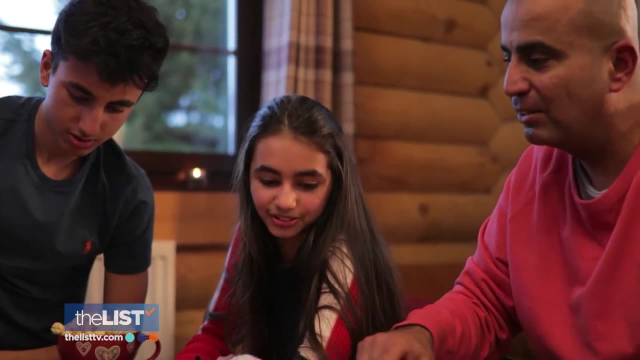 It's time to test, test and test again. Get test players to play your game. It's a key ingredient to knowing that it works. But the easiest test group to gather is the worst one to use. Don't use friends and family to do testing. God bless them. they lie.